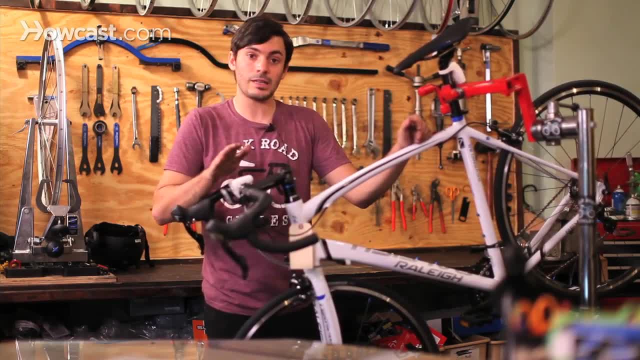 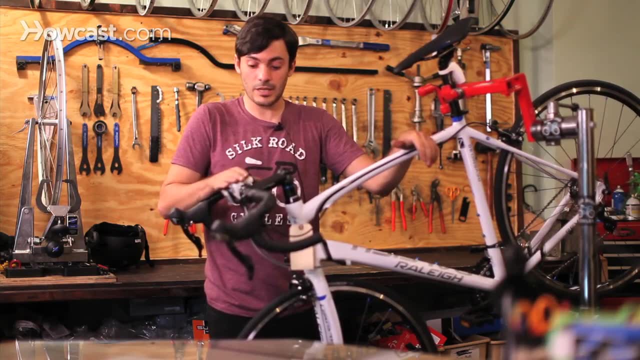 reflectors front and rear, that you have working lights both front and rear- white on the front, red on the rear- just like a car. You can get a pretty substantial fine if you do not have them at night. so basically from dusk till dawn. 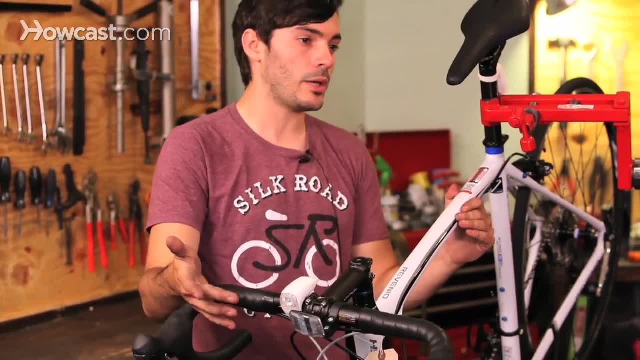 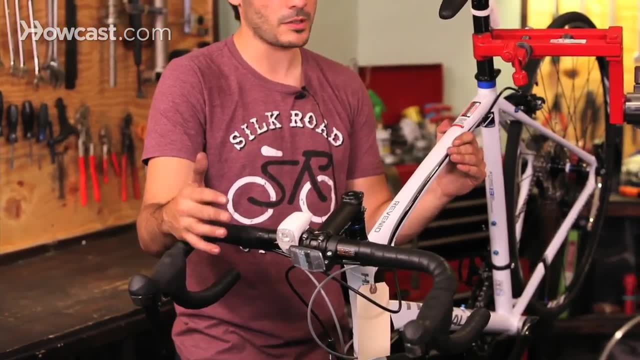 So with lights you have a bunch of different options. Most lights go anywhere from usually around eight dollars on up. They can go very, very expensive depending on how bright they are, What they're made out of all those types of things, Basically for the city, you're. 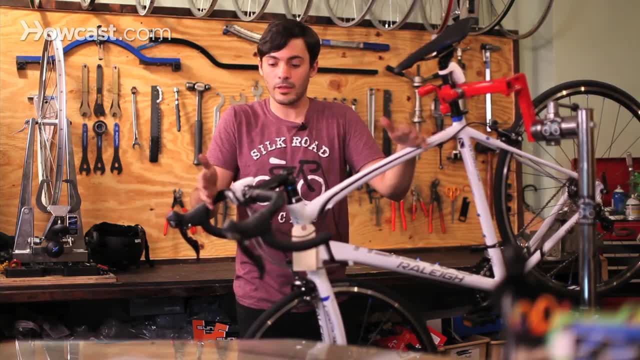 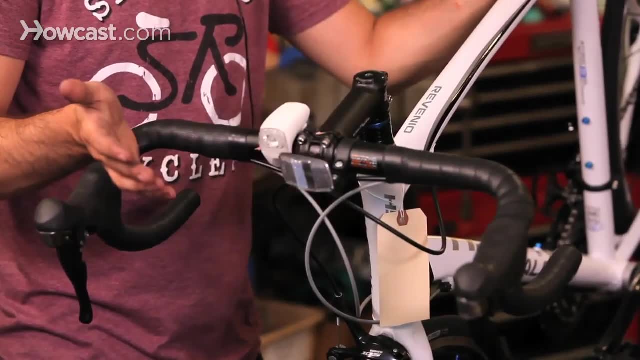 not going to want a light that's going to necessarily illuminate your path. You just want a light that you're going to be seen by cars and pedestrians and other cyclists. So a light like this basically: it flashes, It's nice and bright, It's USB rechargeable. 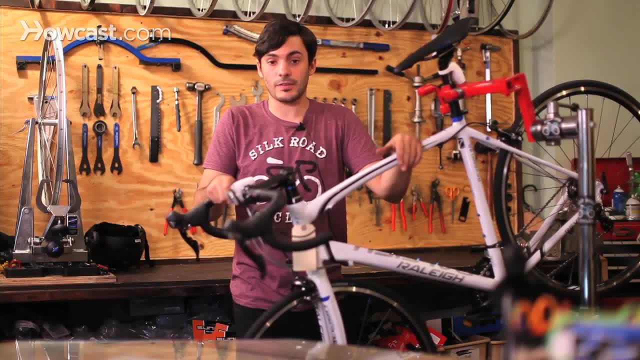 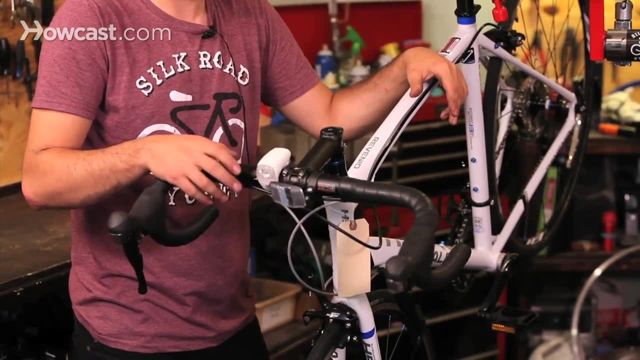 so if you do a lot of riding at night, then you can get this and save a lot of money on batteries. It's just really nice to have in your backpack all the time, just in case you're out and it gets dark. And then the rear one is basically exactly the same: It's going to be blinking, or you. 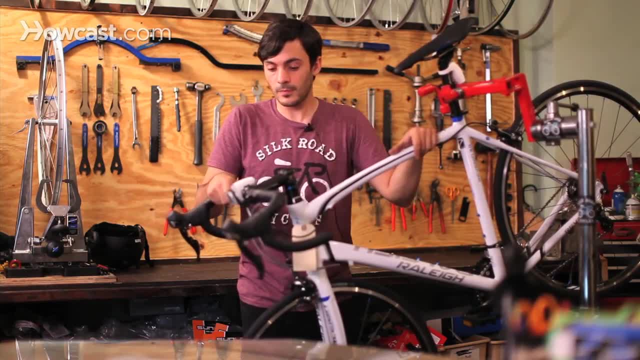 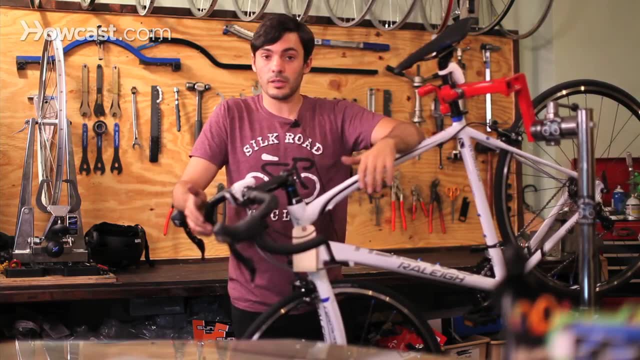 can keep it steady. It's better to keep blinking so people can see you in the city. So that's those lights. Another way to be safe is just to wear the proper clothing and equipment. so make sure that you have a rain jacket with you. if it's going to be raining that day, Make sure you. 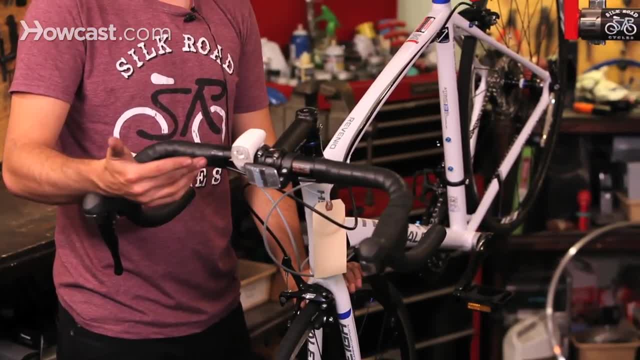 have fenders on your bike if you're going to be riding in the rain or if you're going to be riding maybe in a winter day when there's like slush and snow and things like that, so you're not going to get wet and cold and get sick. 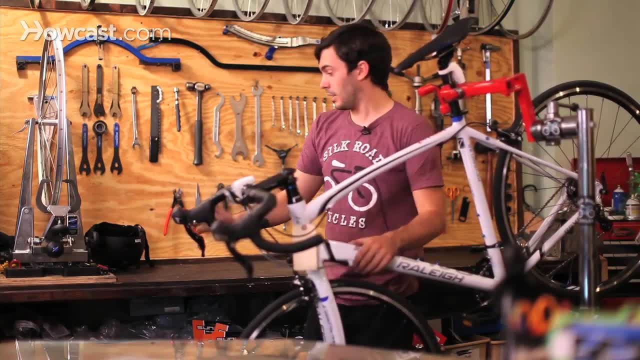 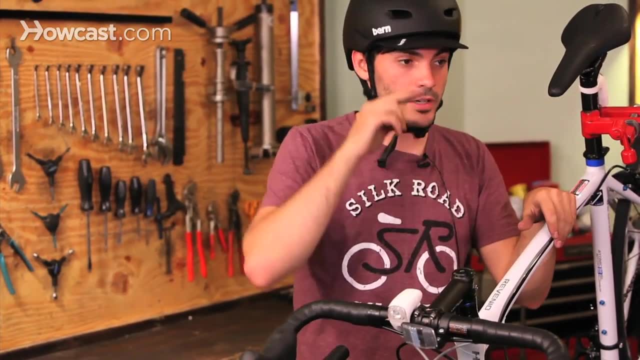 All right, guys. That's it for today. Thank you so much for watching. I'll see you next time. Also, a lot of people don't like to wear helmets, but definitely helmets can keep you safe. Okay, so you want to make sure that you have. You can take two fingers. put it above. 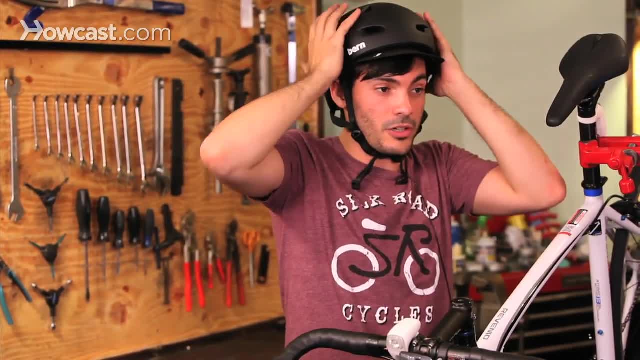 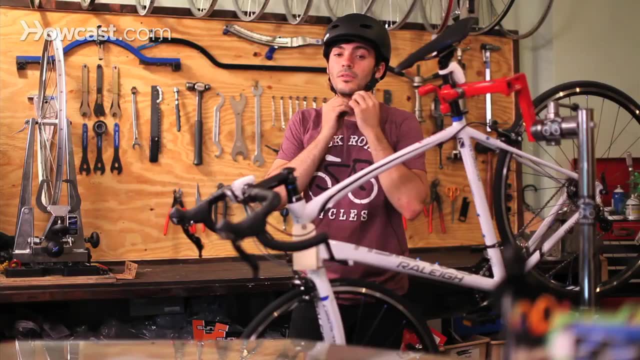 your eyebrow and that's how low the helmet will be. You don't want it far back like that, because then you're going to lose your short-term memory and you also don't want to have it on backwards. So with the strap, you want to make sure that it's fastened correctly and that you can put. 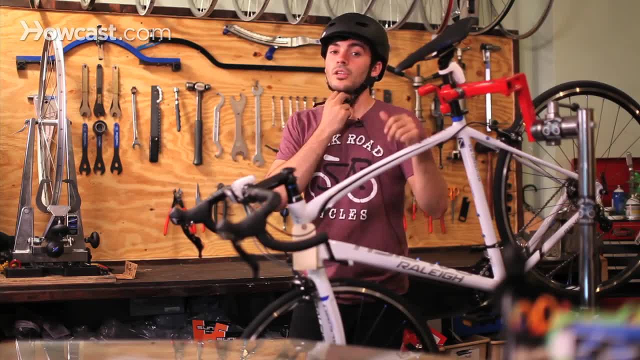 two fingers underneath the strap. This is a little bit loose, so you may want to tighten it up. You just don't want it too tight and you don't want it too loose, because if you hit the ground you don't want your helmet flying off.